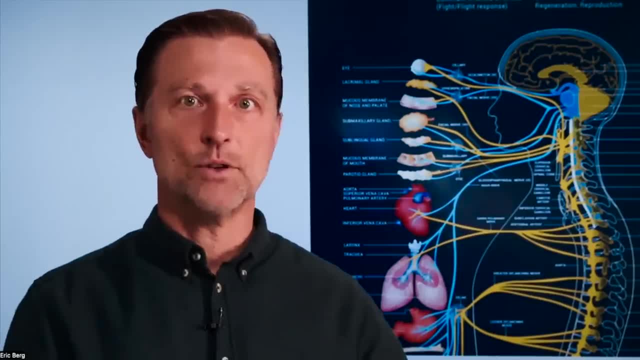 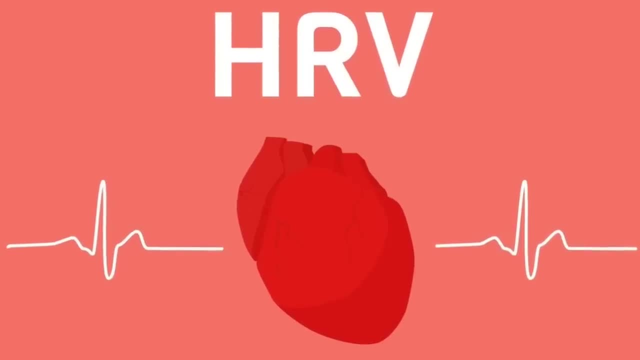 healthy. But if you just barely stand up and you pass out because your body can't adapt to that, you're going to be very healthy, And if you just barely stand up and you pass out because your body can't adapt to that, you're not going to be in good shape. So HRV- heart rate variability- is a technology. 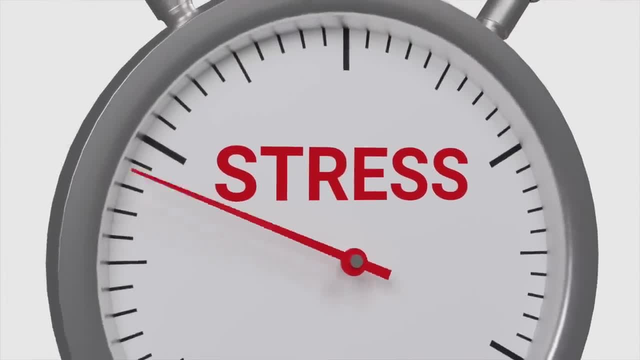 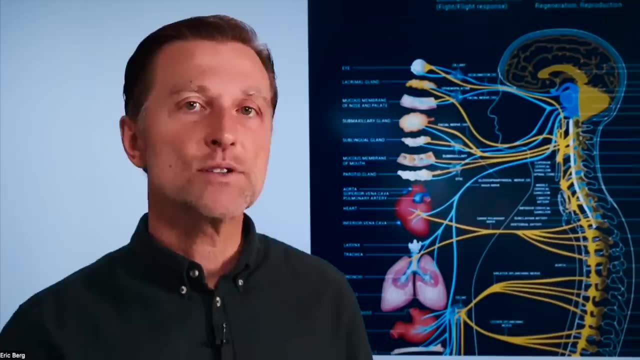 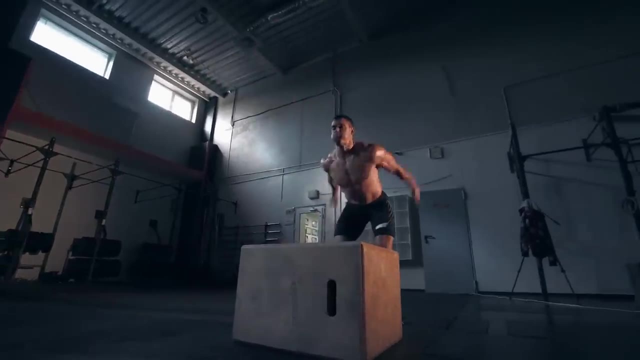 that's very researched. It can help a person understand where they are stress-wise and their ability to adapt to stress, as well as their ability to recover from stress, And a lot of people use this technology in exercise to determine number one: should they work out hard today or should? 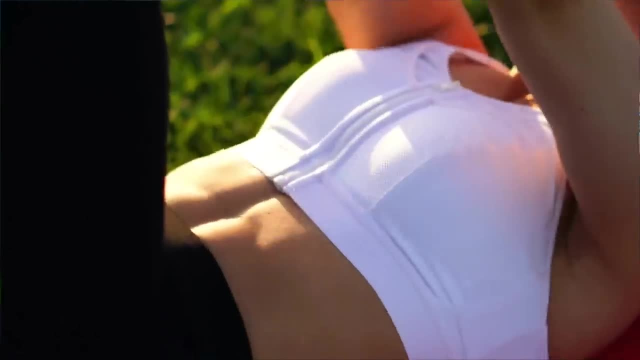 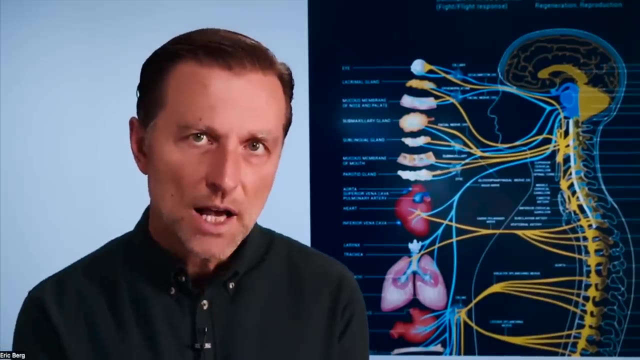 they take a day off, Are they overtraining or do they have enough potential recovery to handle a really good workout? And number two, do they have enough potential recovery to handle a really good workout? There's a lot of lifestyle things that you can do: Food, exercise, activity, sauna. 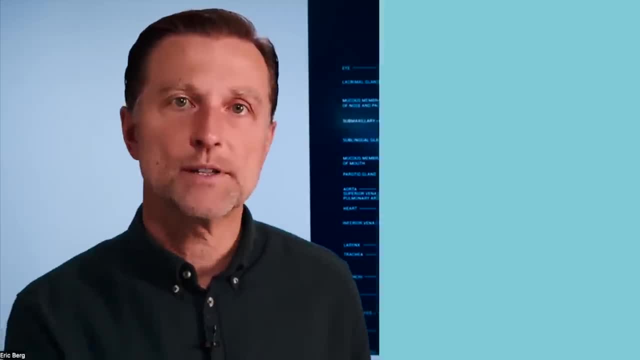 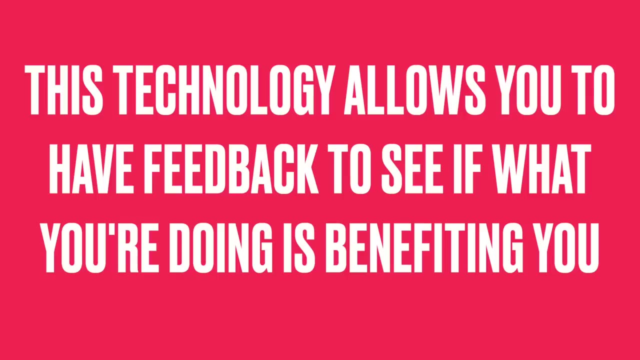 treatments, cold bath, nutritional supplements. This technology allows you to have feedback to see if what you're doing is benefiting you or making you better or not. You basically use this little device that you would put your finger in and it'll pick up information off your heartbeat. 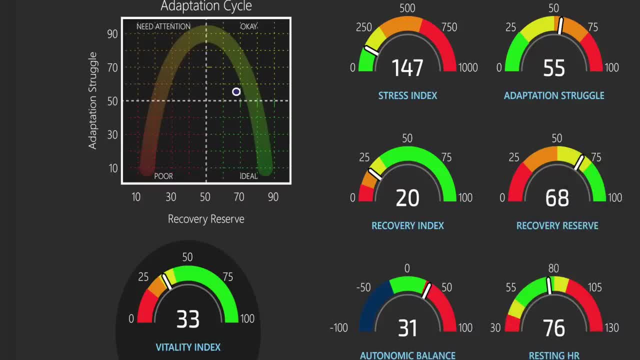 and put it into some software which gives you these graphic illustrations of what's going on with your heart rate, And it'll give you a lot of information about what's going on with your heart stress and recovery, even your biological age. So in practice I would use this on patients all. 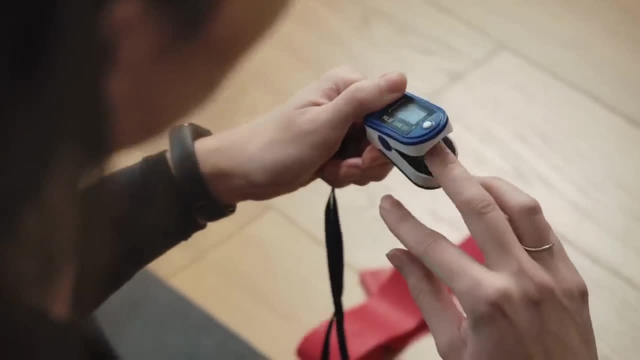 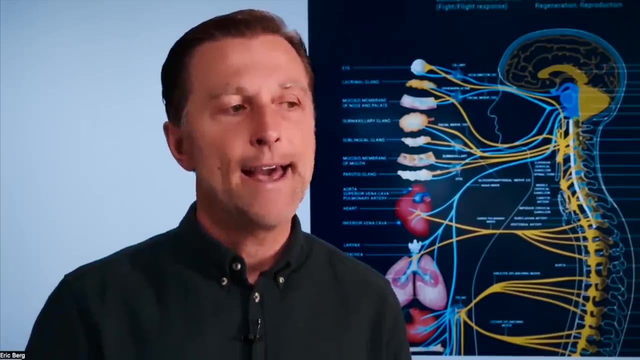 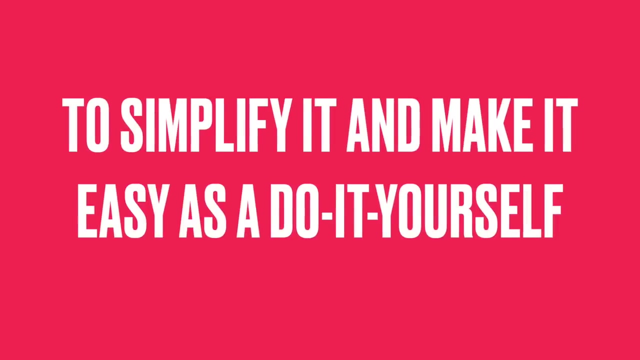 the time I depended on it. It was a really great tool to kind of look what's behind the scenes and see what's happening, And so I recently reached out to the company after probably 12 years of not using it, And they have come a very long way in refining this technology to simplify it, to make 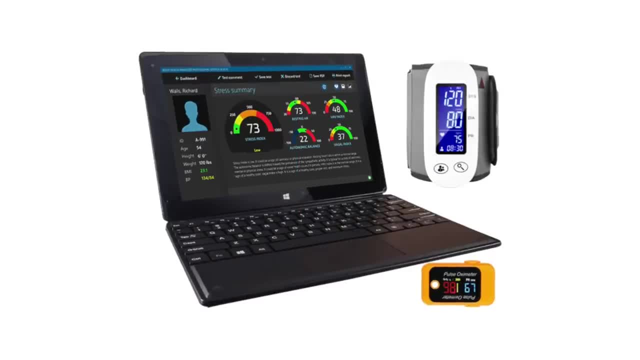 it easy as a do-it-yourself, And so now this device and the software is available to anyone that wants to get it. I'm going to put it in the description box. And I'm going to put it in the description box. Put the link down below. We're done with the video if you want to check it out, But the price is very. 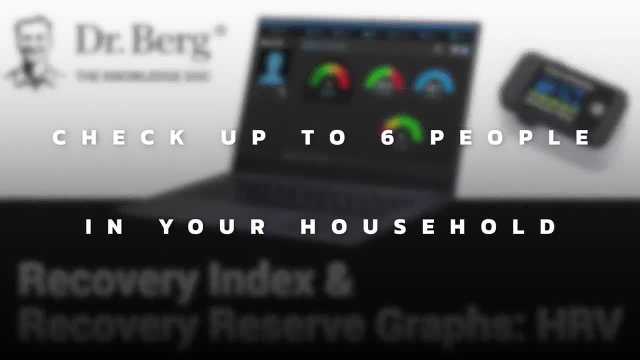 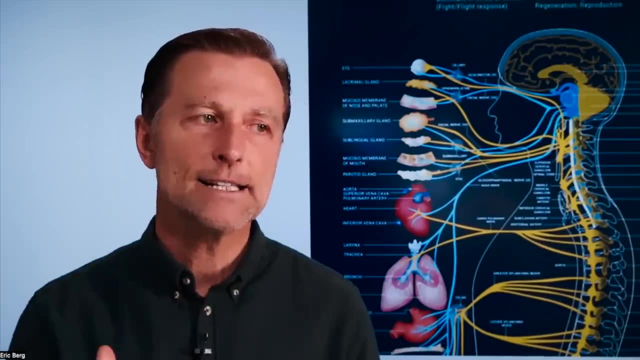 reasonable. You can check up to six people in your household, There's no monthly fees And you pretty much can have your own science lab to figure things out, Because you really can't take things to the next level, improve things if you can't measure it. So anything, you have to measure it, whether 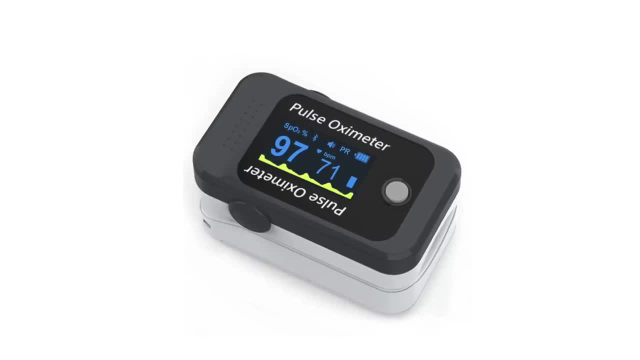 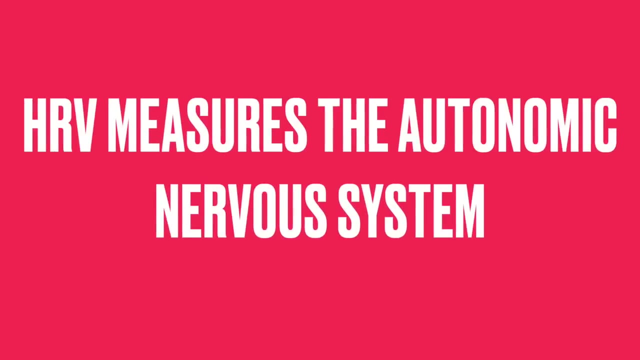 it's a blood pressure cuff or a pulse rate or whatever. if you can measure it, then you have this feedback tool to see if what you're doing is working or not. Heart rate variability measures the autonomic nervous system. right here, The autonomic nervous system is the system. 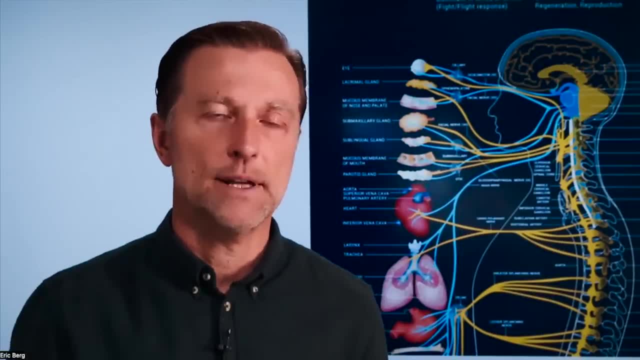 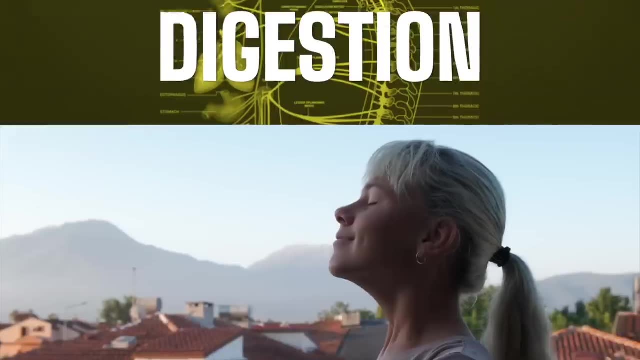 that works on automatic, that you don't have to think about it. It's involuntary. So this includes blood pressure breathing digestion. Now, of course, you can control your breathing, but then, if you forget about it, you'll still keep breathing. So there's an involuntary component to this. 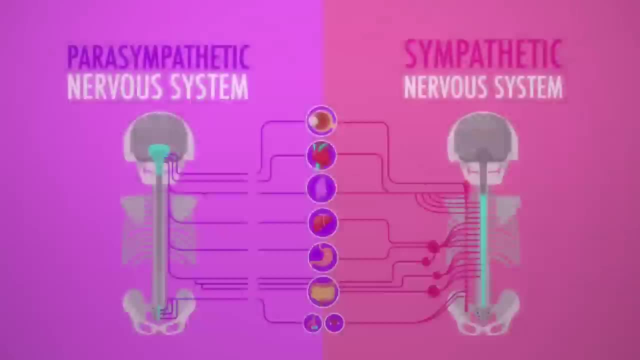 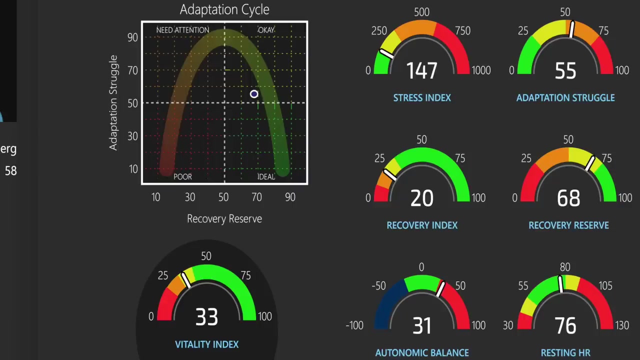 There's two branches. One is the sympathetics, which is the flight or fight, And the second one is the parasympathetics, which is the rest and digest. We didn't name it sympathetic and parasympathetic, We named it stress index. 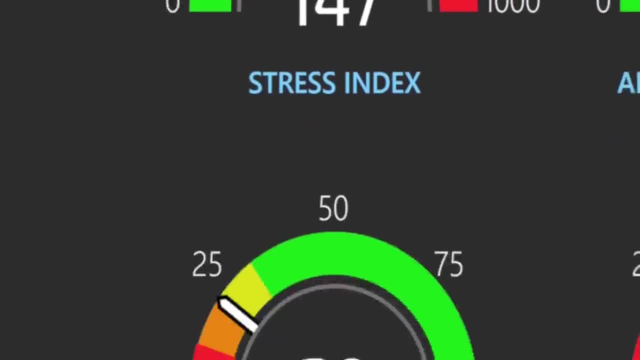 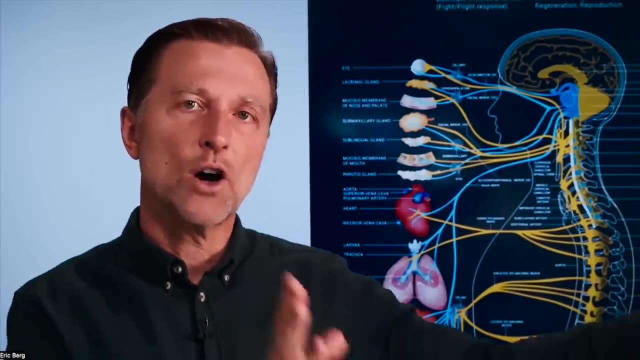 which is your ability to adapt to stress, And then we named it recovery index, your ability to recover from stress. So the simplicity of this is that HRV is the tool to measure the autonomic nervous system, which controls a lot. as you can see right here, Every tissue in the body is 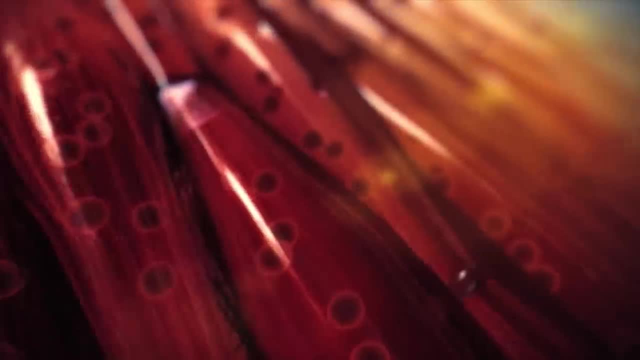 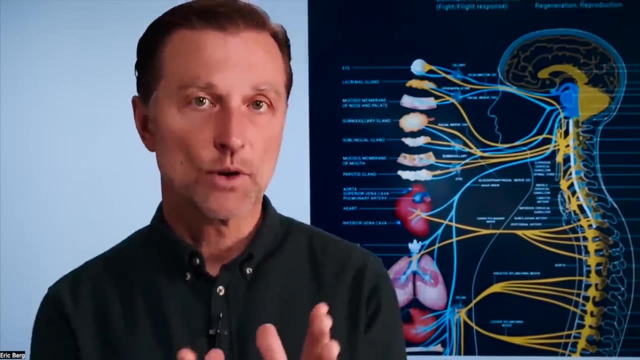 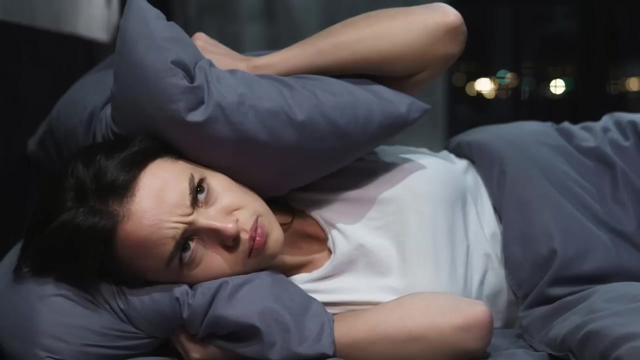 controlled by it. And so this is a window to look inside your body to kind of see the state of where people are heavy on the stress or sympathetic mode or sympathetic dominance and they're low in the recovery or the parasympathetic. So this kind of explains why they can't sleep. This is why. 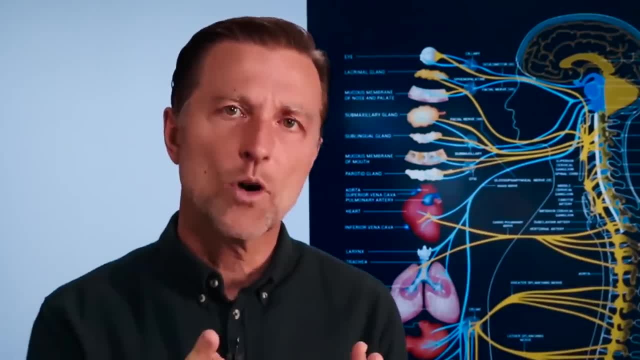 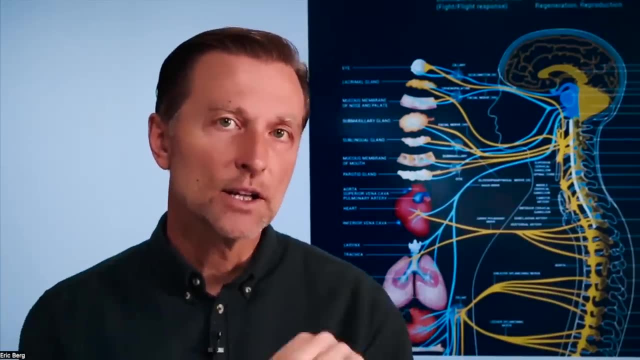 they're stressed, But I created a lot of videos to understand this a lot more and how to use this and then what to do to improve these graphs. And even if you don't get this device, I'm going to include the training videos down below so you can check them out, because there's a lot of great data. 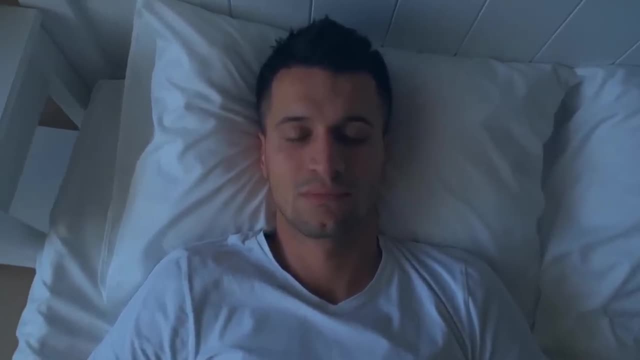 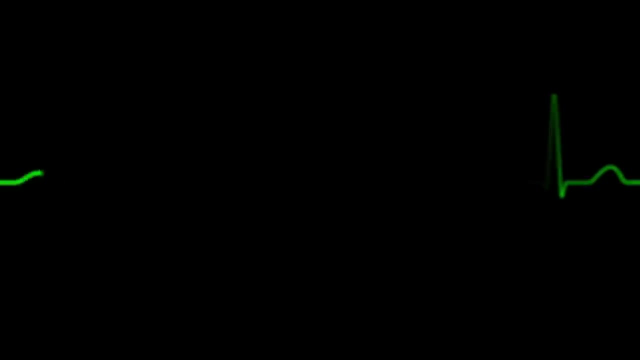 that I put together. I'm going to give you one example. I'm going to give you a little bit of a example. Let's say you go to sleep at night and you have a hard time going to sleep. Well, the parasympathetic nervous system, the recovery system, is always active and it's pushing your pulse rate. 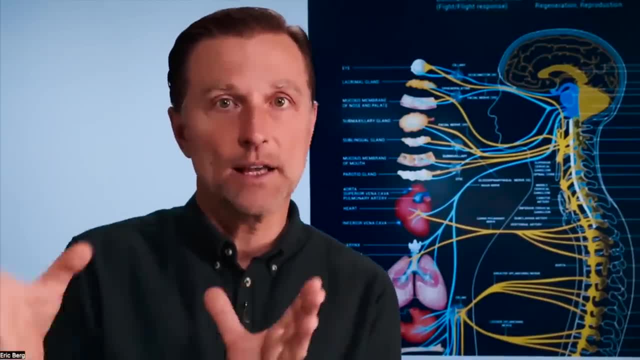 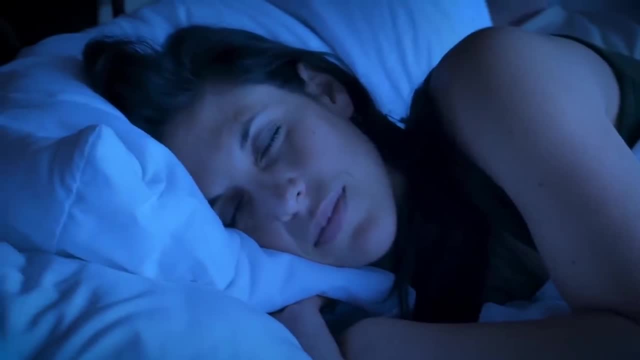 down And if that's weak, okay, and then you're also heavy on the sympathetics, the flight or fight, then you're going to have a hard time going to sleep. So you'll just lie there and your body won't turn off. So that parasympathetic is the system that pushes you into the deep delta wave. 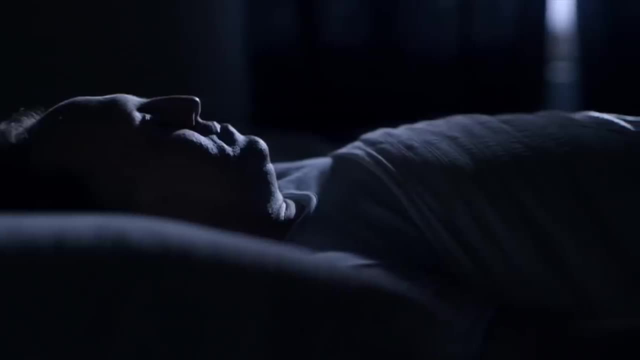 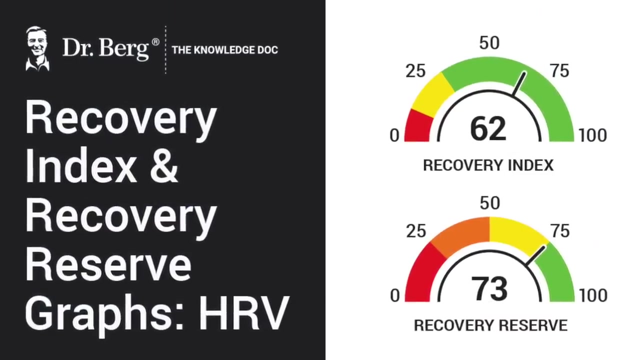 non-REM phases of sleep where you're rejuvenating and you're recovering all the body functions. So you'll see when you take the graph, if you can sleep good then you'll see that graph will correlate. If you don't sleep good, that graph will not look very good. And then the second half. 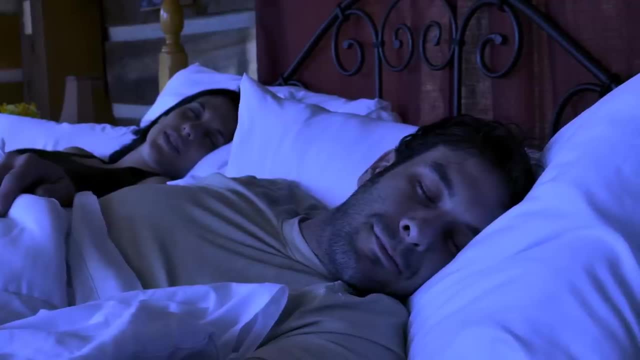 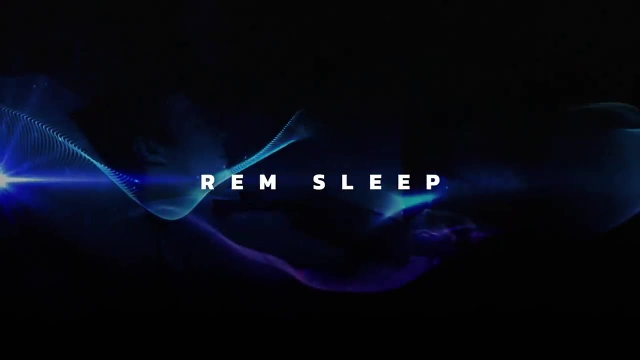 of the sleep is kind of controlled more by the sympathetic nervous system And this is why, kind of like, the wavelength REM sleep is a very active wave, similar to when you're awake but you're actually asleep. So if you have a problem with the sympathetic nervous system, you may find 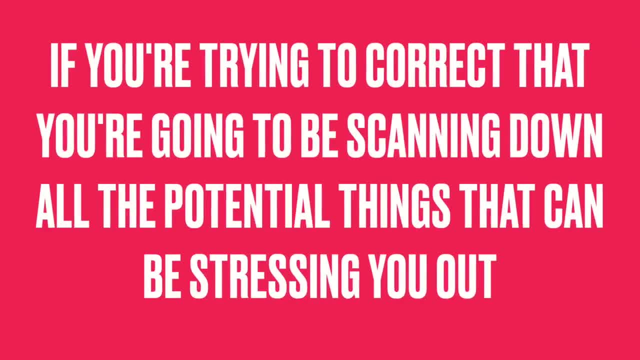 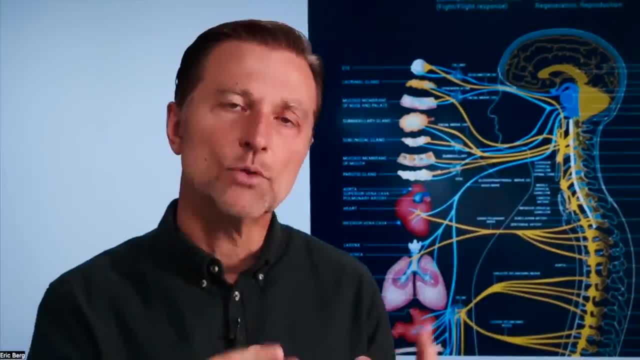 that last bit of sleep, that REM sleep. So then, if you're trying to correct that, improve that, you're going to be scanning down all the potential things that could be stressing you out And then you'll chip away at that And then you'll retest back and forth to see if it improves to really 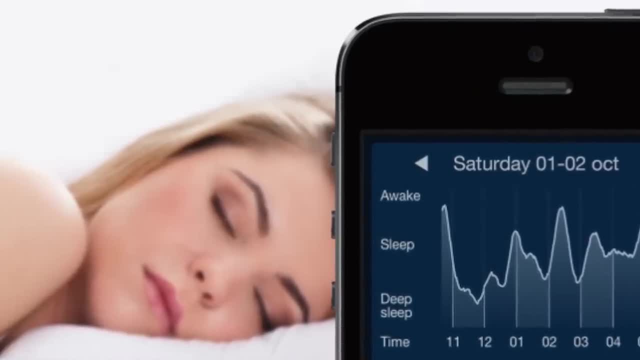 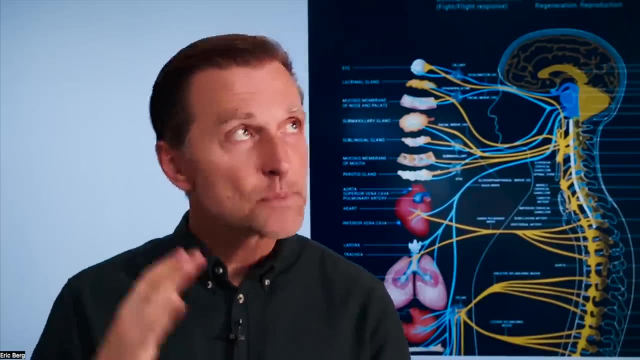 see if that was the thing that was causing most of this problem. There's also another great tool to help you not overtrain. I'll give you an example. When I train hard and I sprint up like a mountain right And I'm just like pushing myself And then I recheck my biological 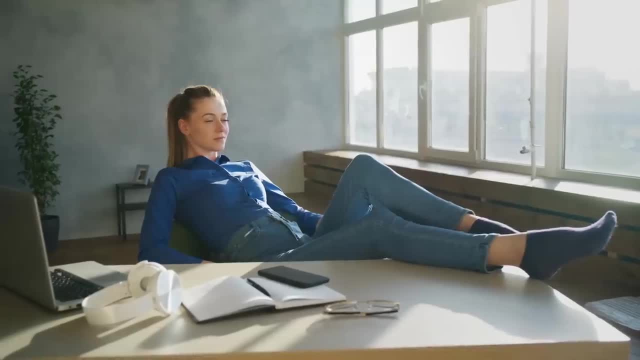 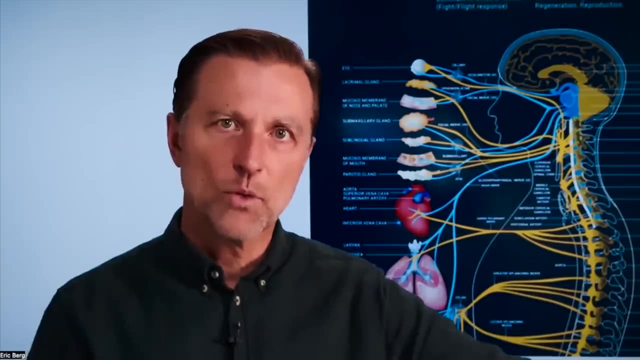 age the next day. I'm like 80 years old, So that kind of tells me that I should probably take a day off, right, And just rest, And then I'll check on the next day and see when it comes down, and comes down to the point where I'm safe to actually do that again, Whereas before, when I didn't have. 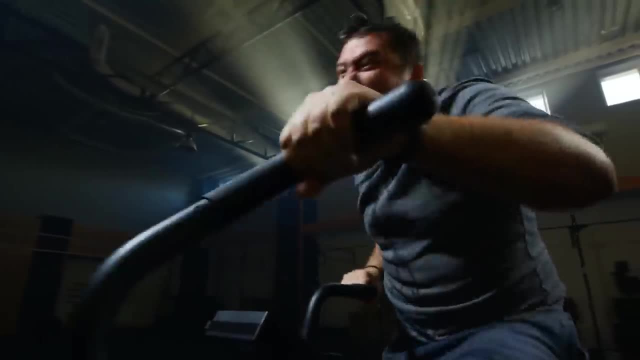 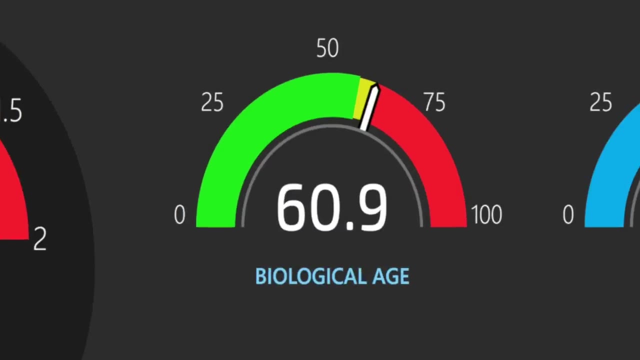 this technology, I would tend to push myself a little bit harder than I should and overtrain and wonder why I had more inflammation and had other issues. And one really cool thing about this is biological age right. You're able to look inside your body and see the age. 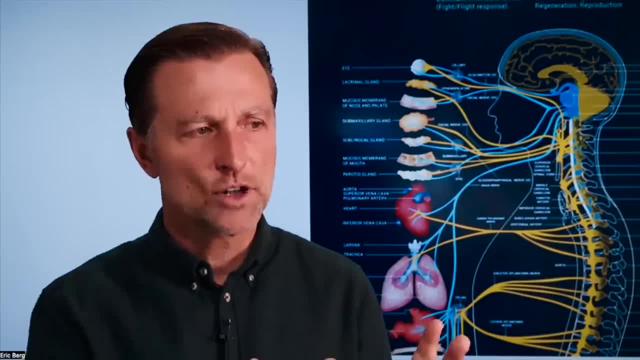 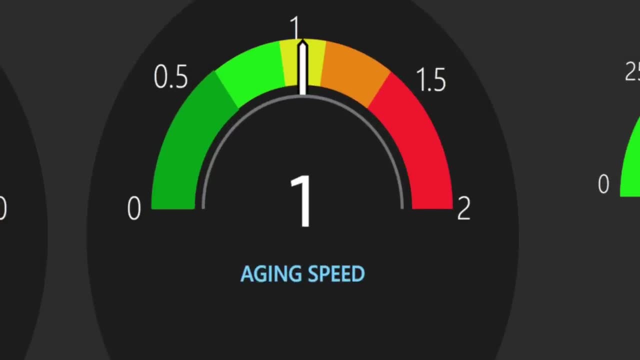 of your cardiovascular system and arteries. You're able to determine how elastic and how resilient they are. You can also measure the rate of aging, which is a really cool graph too, And there's a lot of things that can improve this graph and make it worse too, Like it'd be a really 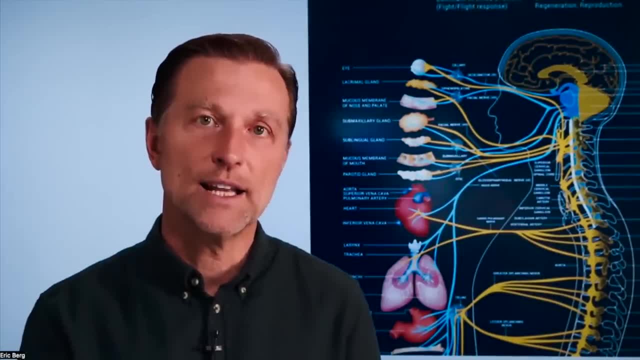 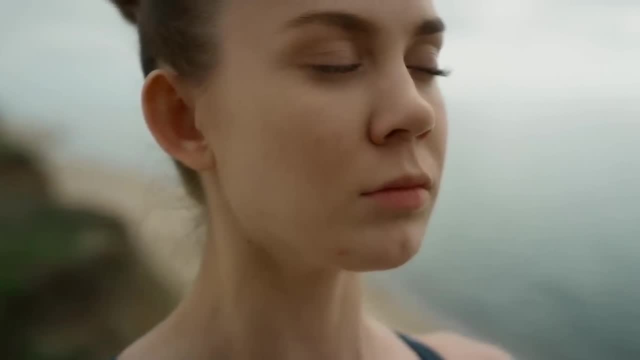 great experiment to have you go out drinking one night and then do a before and after the graph. You'll see big changes. There's all sorts of training on just breathing exercises that you can dramatically improve your graph. So I just wanted to introduce you on. 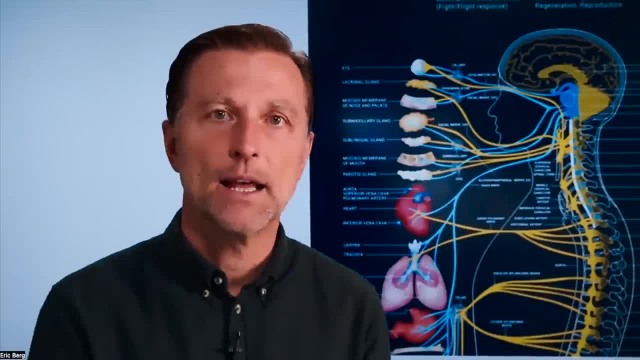 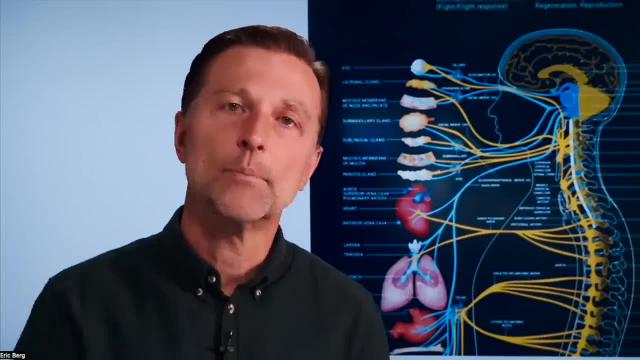 this technology, heart rate variability and exactly what it does, And it measures your autonomic nervous system- And if you'd like more information about this or would even like to see the training videos, I put that down below. Check it out.